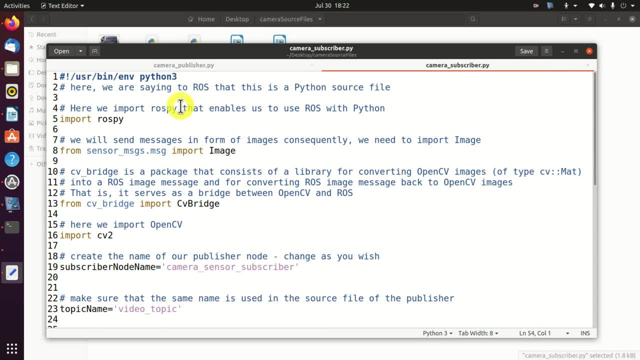 In this video tutorial, you will learn how to write these codes from scratch and how to build a ROS package that will govern the whole process. But before I start, I would like to provide the answer to the following question: Why is this video tutorial relevant? Well, this video tutorial is very important for 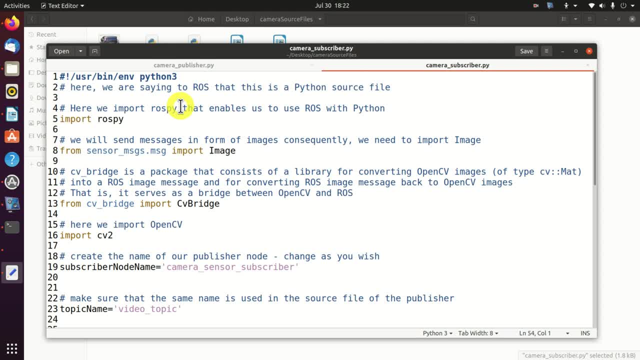 machine learning, computer vision and robotics applications. Namely, you will use a camera to detect objects or to perform some kind of motion planning, analysis or obstacle avoidance, And you need to know how to integrate camera reading with ROS and OpenCV. Eventually, you 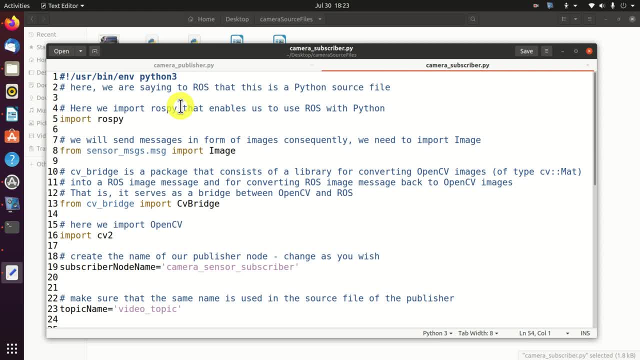 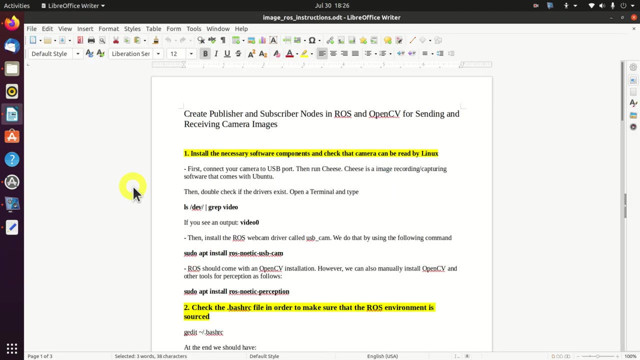 will perform in OpenCV some image processing or segmentation, contour recognition, object recognition, and then you will couple OpenCVs with the ROS package. You will be able to see the results of these models in the next video tutorial. Thank you. Also, before I start, I would like to mention the following: It took me a significant amount of time, energy and planning to create this free video tutorial, as well as almost 300 free video tutorials that you can find on my YouTube channel, And consequently, I kindly ask you to press the like and subscribe buttons. Thank you. 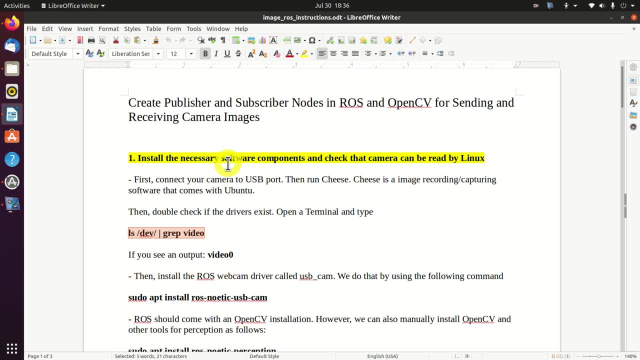 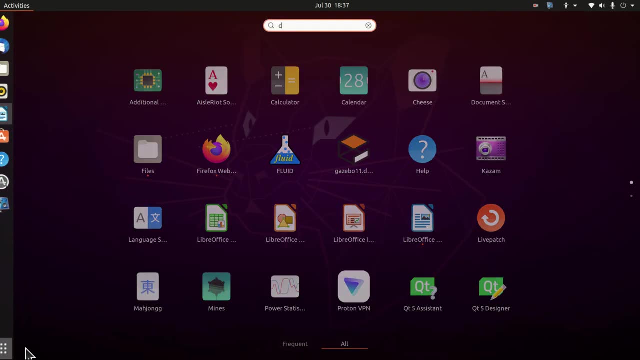 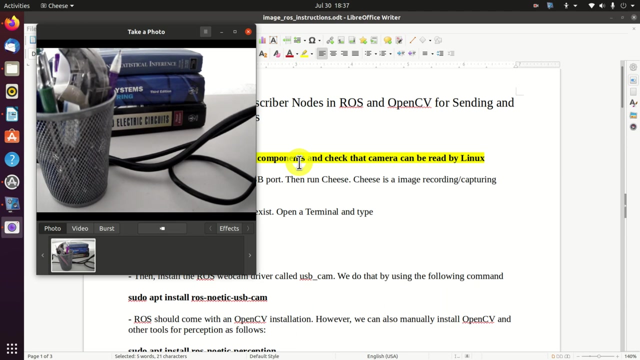 Alright, let's start. The first step is to install the necessary software components, and check of their camera can be recognized by Linux. Let's do that. First, connect your camera to the USB port, Then open this program called cheese. Cheese is the free software for taking images and recording videos, and it comes with Ubuntu. 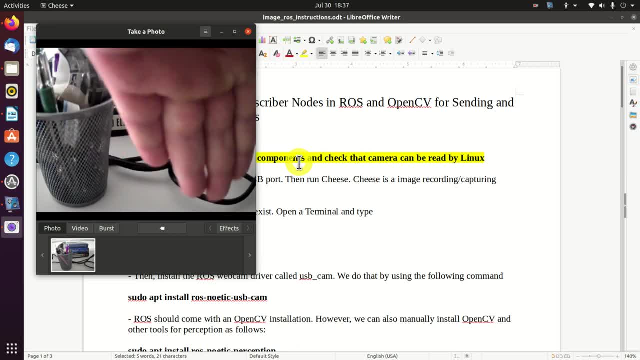 Okay, this is a image And I can see it There. it is There, it is. Look what I find here. First, an image: it's here. Okay, can see my hand over here moving. this means that the camera is working. however. 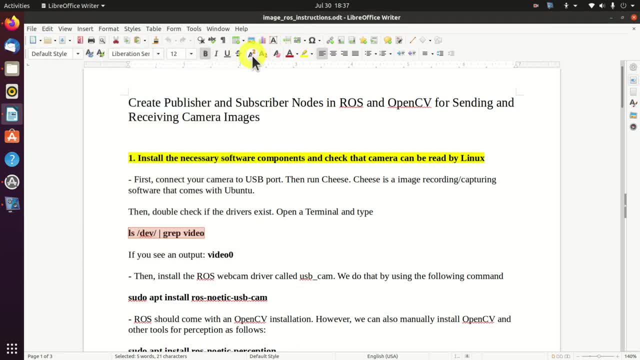 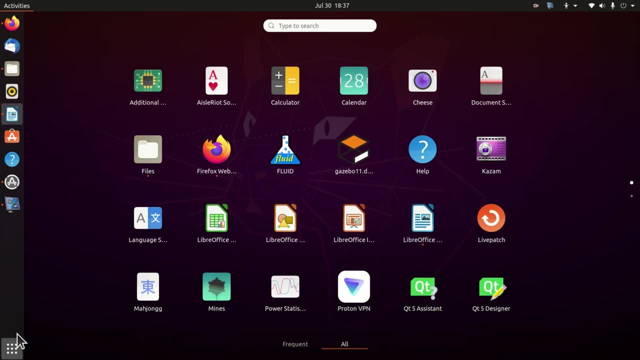 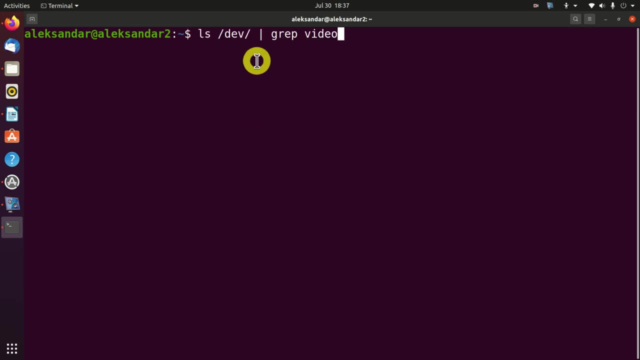 we still need to perform a few other checks. first of all, we need to check the drivers from our terminal. let's open a terminal or here type terminal, and inside of the terminal let's type this command: we see video zero and we see video one. video zero is the device that corresponds to the default camera and 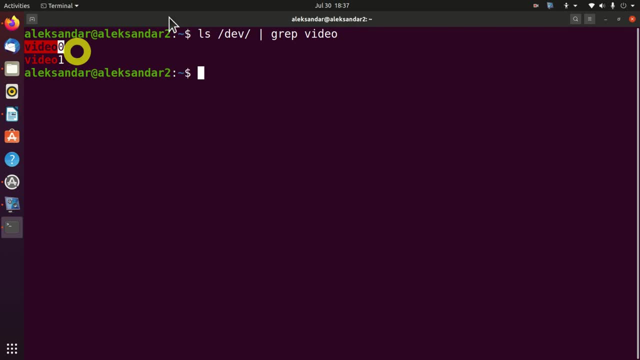 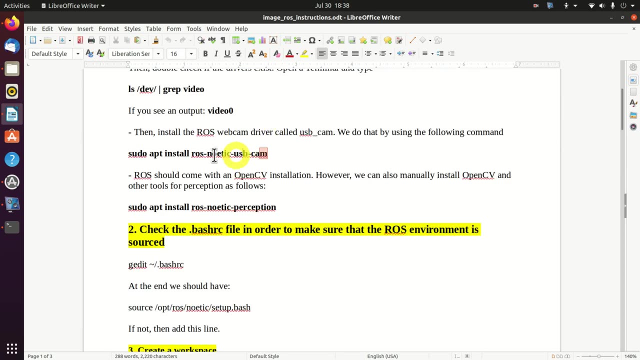 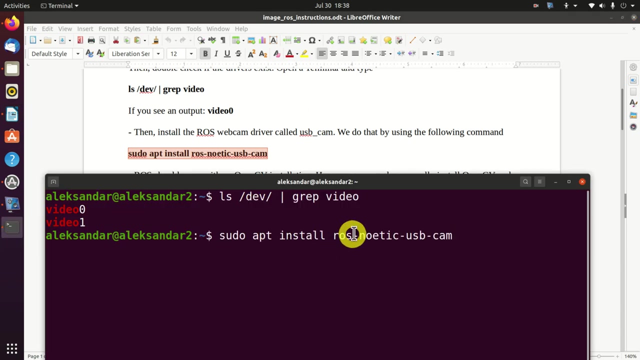 consequently, this is a good sign. let's continue. the next step is to install the ROS drivers for our camera. to do that, we will use this command: sudo apt. install ROS noetic USB cam. notice over here that I'm using ROS noetic distribution and my advice and strong suggestion is to install this version of ROS. let's see. 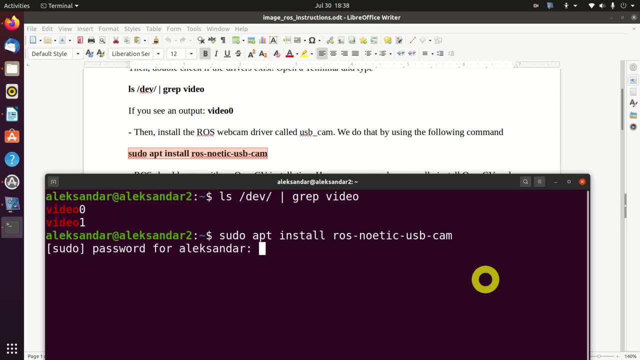 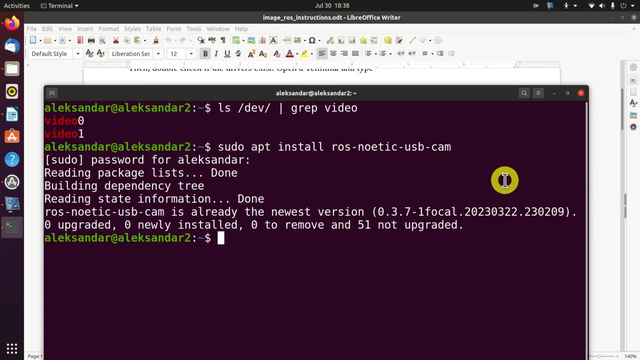 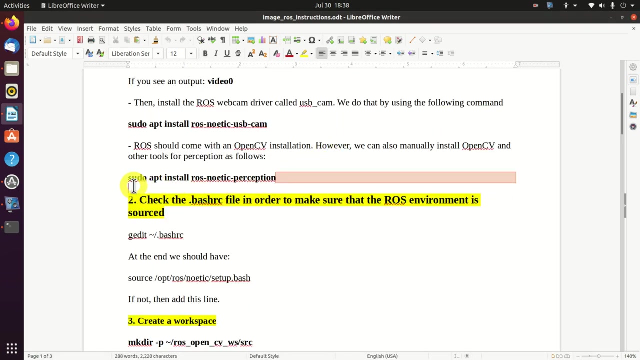 what will happen and, of course, everything is already satisfied, since I pre-installed all the drivers. however, in your case, you will most likely see an installation progress over here and after a few seconds, everything will be completed. good, let's continue. usually, OpenCV comes with ROS. however, maybe while installing ROS, noetic. 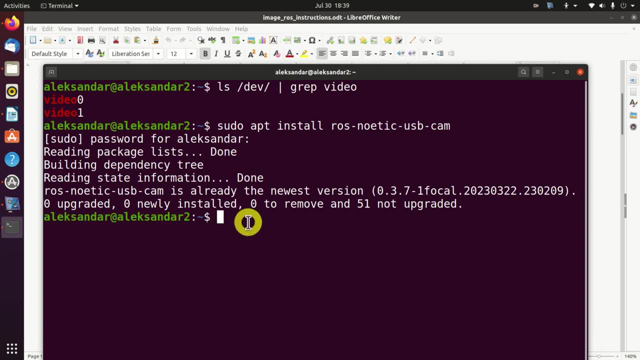 distribution. you made an error and OpenCV is not installed and consequently it's a good practice to verify that OpenCV is installed. the best strategy to do that is actually to try to install OpenCV. to do that we type: sudo, apt, install ROS noetic perception. this library, or this package, contains not only 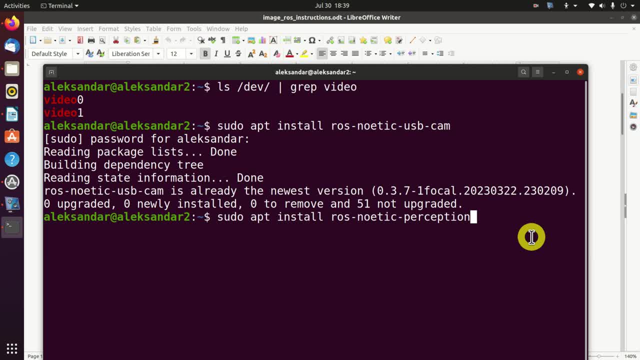 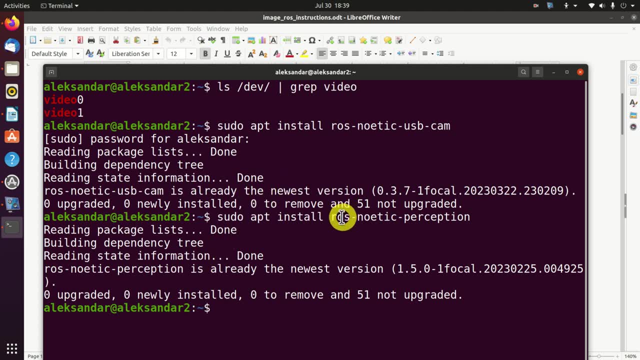 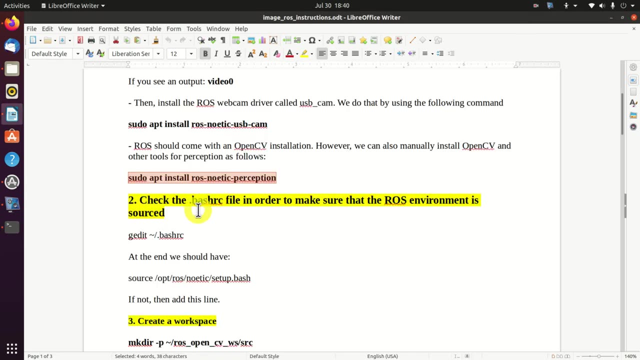 open CV, but it also contains other program programs for perception and you can see that basically all the requirements are satisfied. this is because I already installed this package. so far, so good. next, we need to verify our dot bash RC file in order to make sure that the Ross environment is. 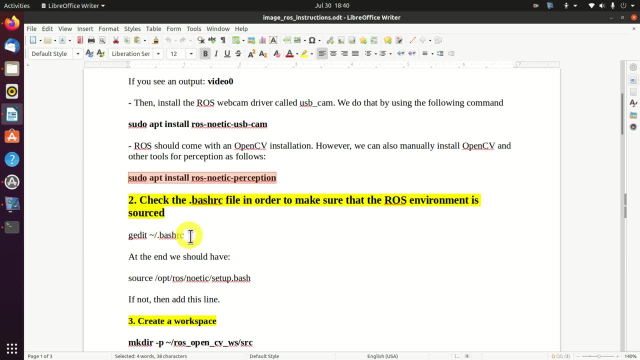 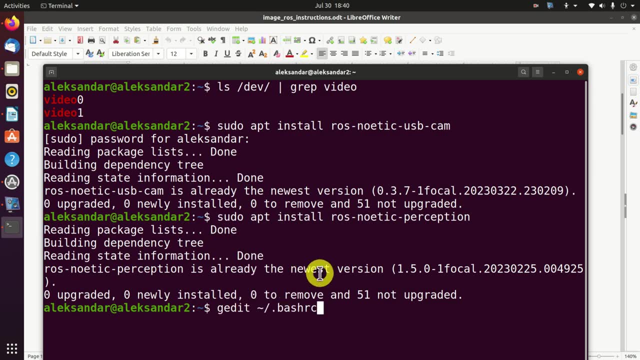 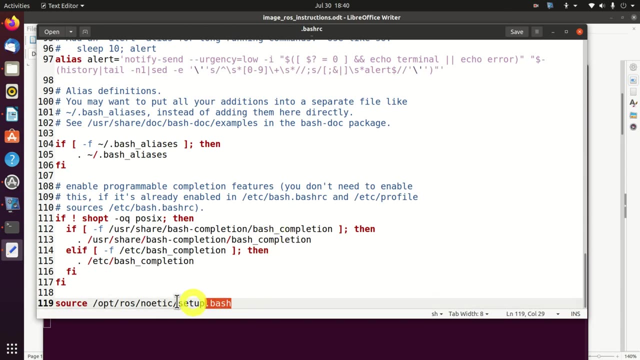 properly installed and source. to do that, we need to open the file dot bash RC. so let's do that and let's inspect the file. here's the file. at the end of this file you should see this line: if your Ross environment is properly installed, this command will simply source this script and it will execute this script. 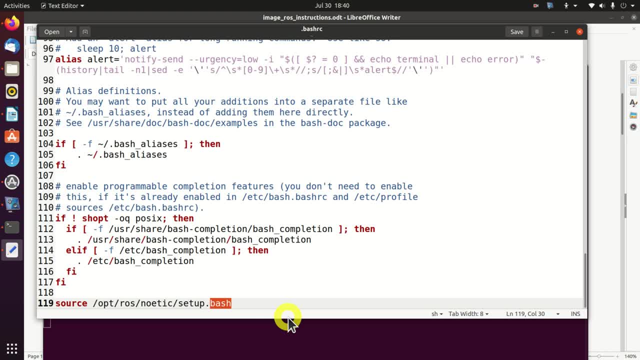 every time you basically open a terminal, that is, after you open the terminal, this command will make will ensure that Ross environment will. Once you open recipesdk, you can see that tisel is now totally is probably is properly being set up. okay, we have this line. if you don't have this line, 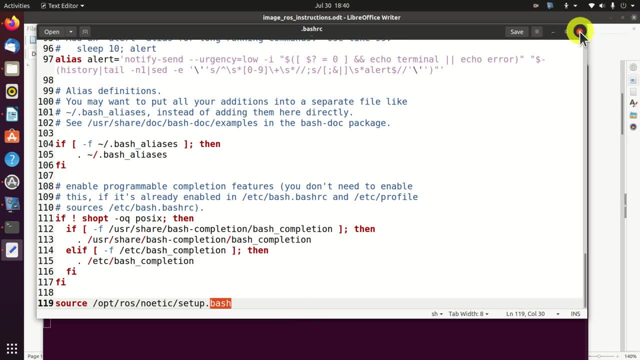 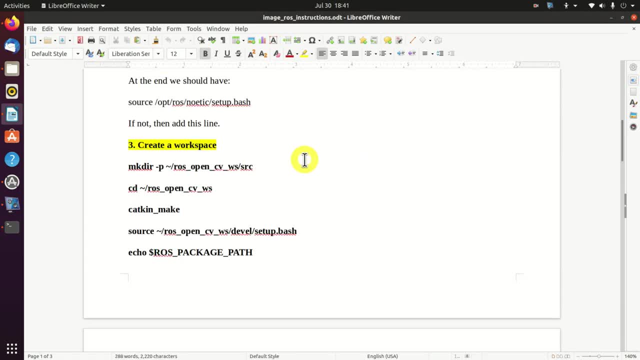 simply type this line at the end of the bash rc file. so far, so good. let's continue. the first step is to create a workspace. to create a workspace first, we will create one folder called ross, opencv ws. you can name this folder as you wish, and inside of this folder, 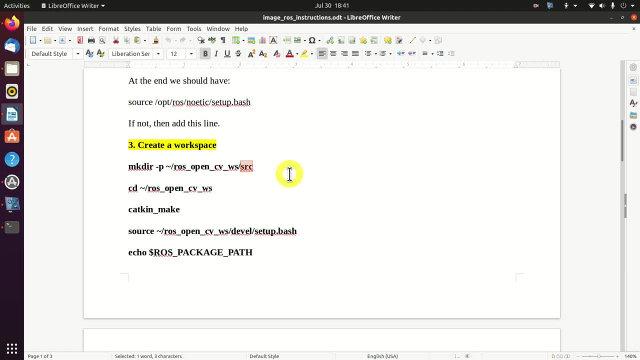 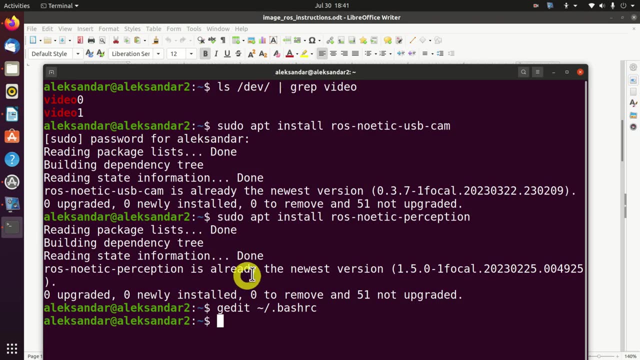 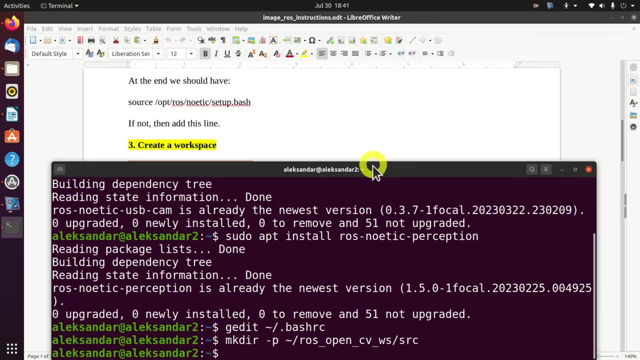 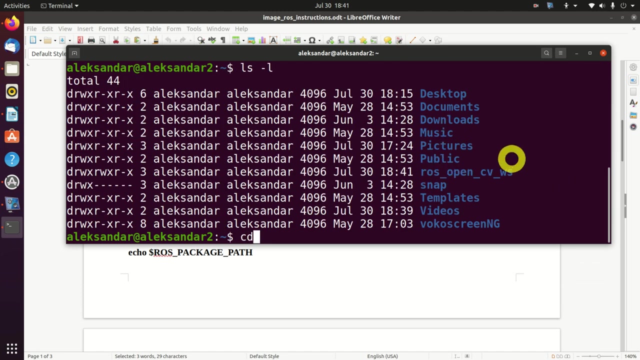 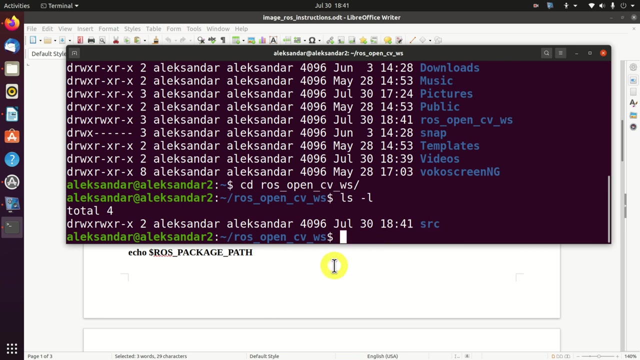 it's very important to create src folder or the source folder, so let's do that and let's inspect the newly created folder. here it is. let's move to that folder. okay, we can also see the source subfolder to create our workspace. we use this command catkin make, so let's do that. 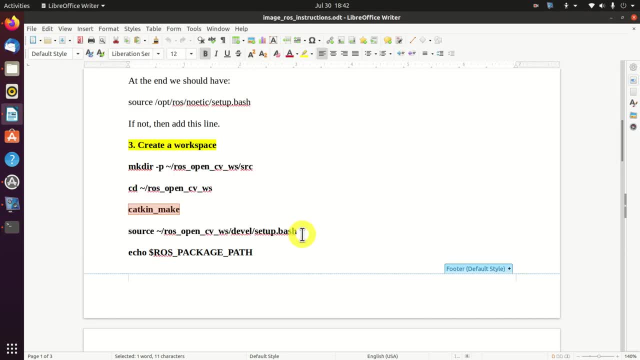 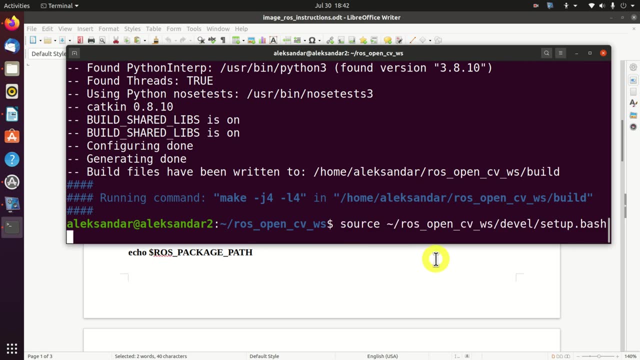 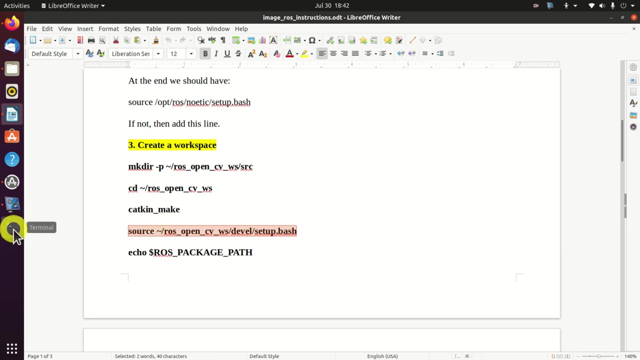 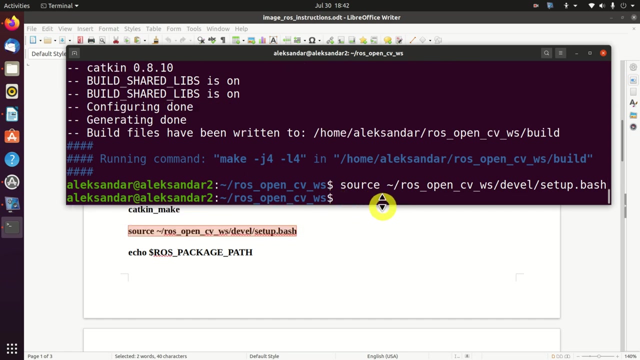 okay. next we need to source this file over here. consequently, we will type this command: make sure that you probably entered properly, entered everything. it is probably entered. let's verify that we have probably properly sourced our environment. we will type echo and then we will type ross package. 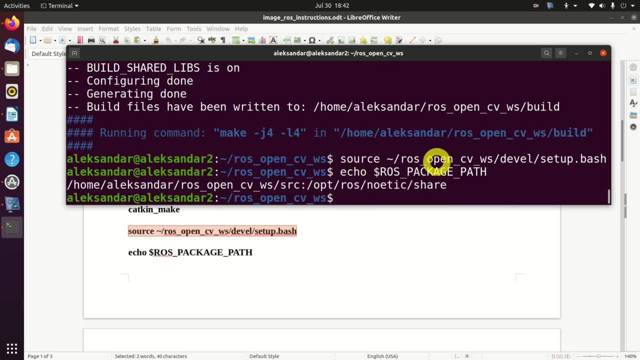 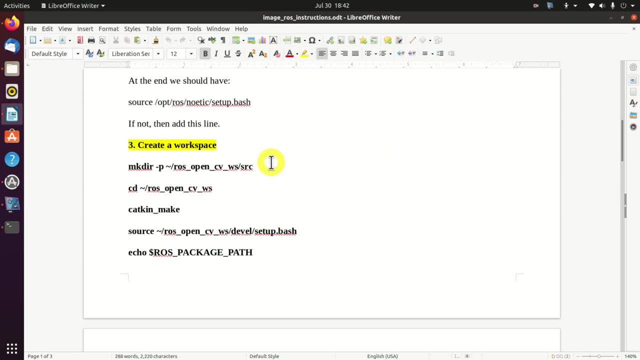 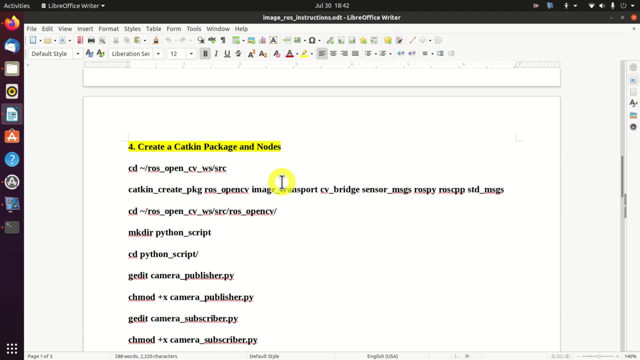 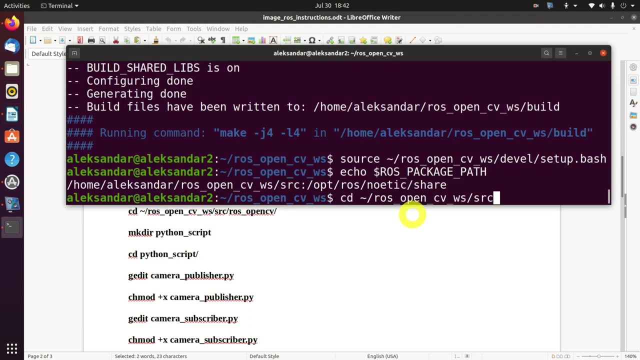 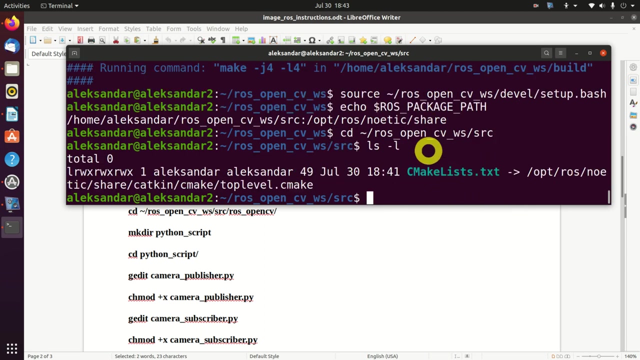 that is, we will inspect this variable ross package and over here we can see the correct path to our newly created workspace. so far, so good. let's continue. the next step is to create our catkin page package and nodes. first we will move to this folder. let's inspect the folder. here it is. let's see how to create the package. 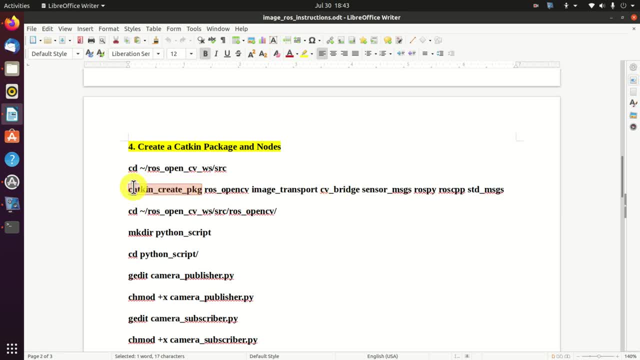 to create a package. we use this ross command, catkin: create package. then we specify the name of the package. in our case it's ross opencv. however, you can change this name, and over here we need to specify the dependencies. we have one, two, three, four, five, six dependencies. dependencies are ross. 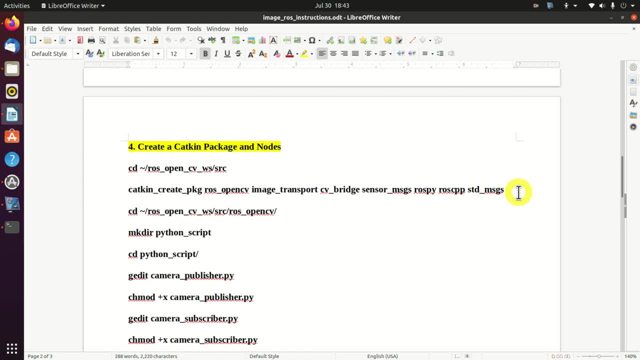 packages that we will automatically import in our new package. this package is used to transport images. this package is used to convert opencv images to ross messages and vice versa. this is the standard package for sensor messages. this is ross pi package necessary to run python codes. 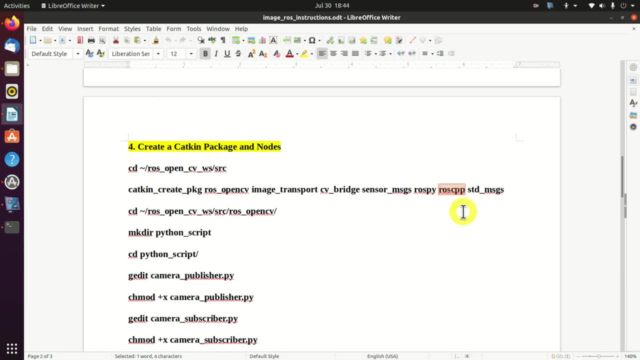 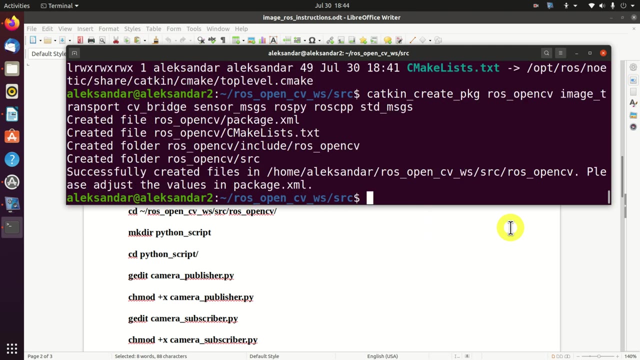 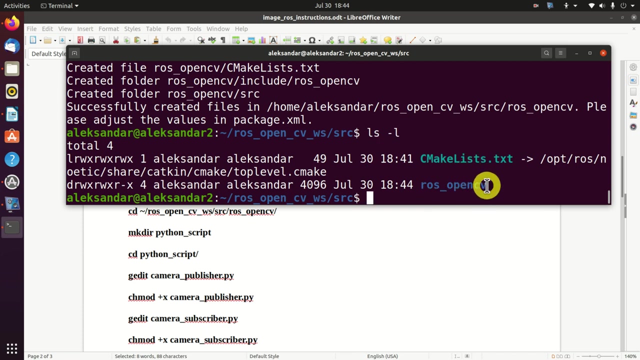 this is ross cpp package. use to run c plus plus code and this is the standard message package. okay, let's create our new package. so far, so good. let's see the structure of our folder. over here we can see our new package. let's go to our new package. 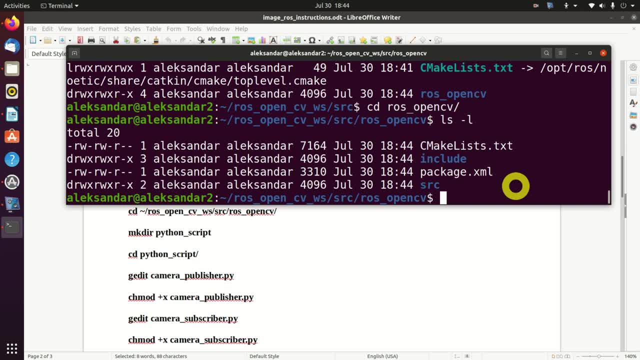 and let's see what is inside. Aha, We have CMake lists, we have include folder and we have two additional objects such as this: one packagexml file and the source folder. Next, we need to create a folder in which we will store our Python. 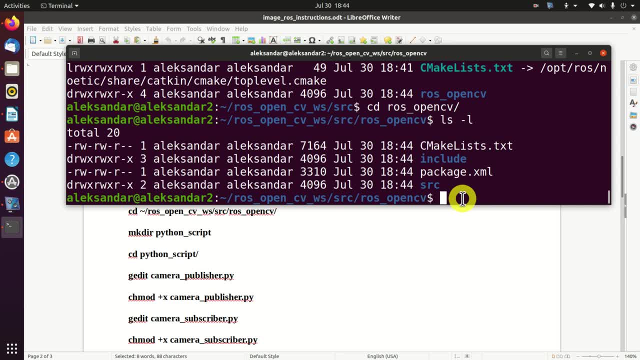 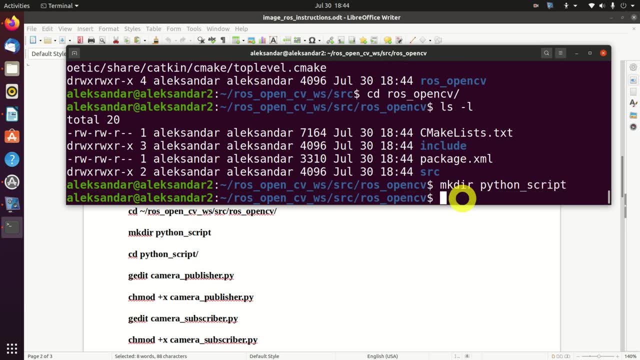 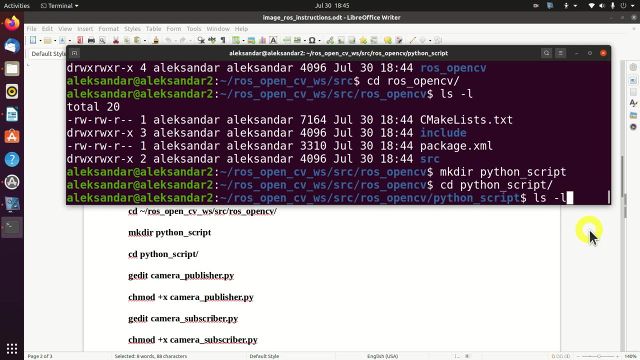 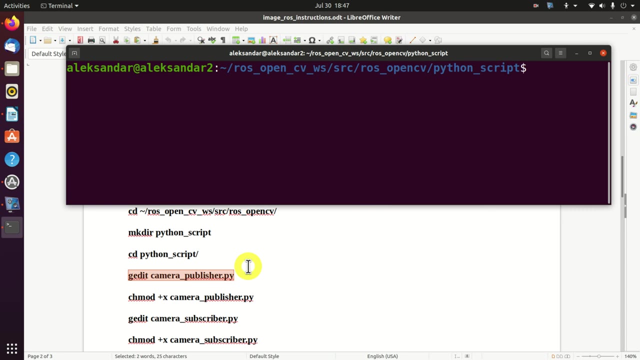 scripts, that is, the scripts for our publisher and subscriber notes. We will call this folder as Python script Here. we created this folder and let's go to this folder. Of course, the folder is empty. Next we need to create a source file that will implement the camera. publisher. Let's do that. I will call the. 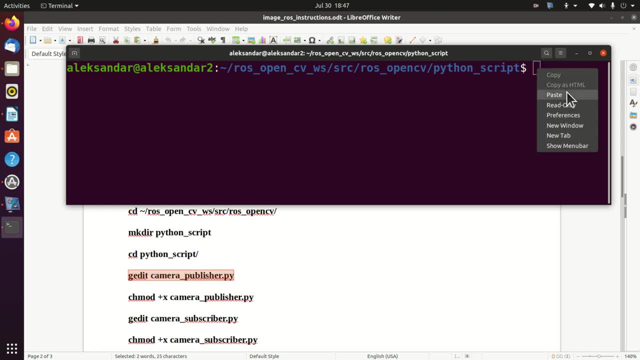 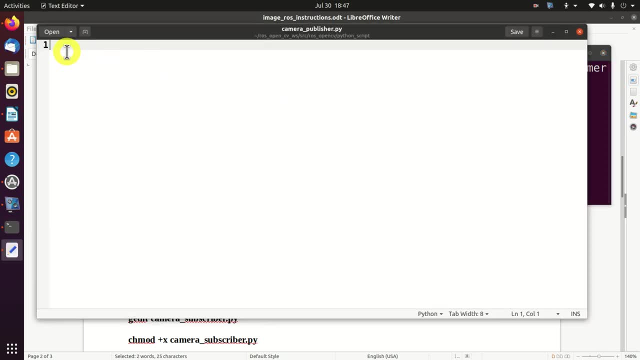 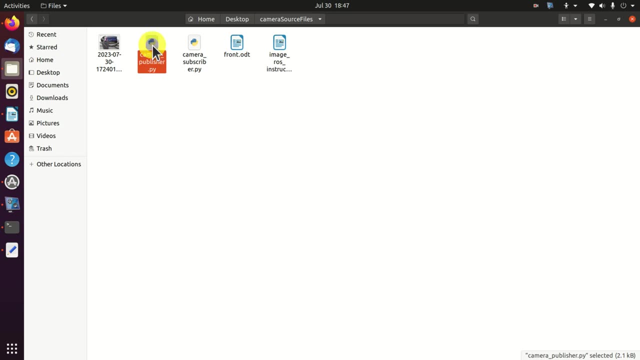 file as camera-publisherpython and I'm using the g editor to edit the file. Here is the empty file. Here we will type the Python code. However, in order to make this video as short as possible, I will simply copy and paste the pieces of code that I wrote previously, And here is the file. 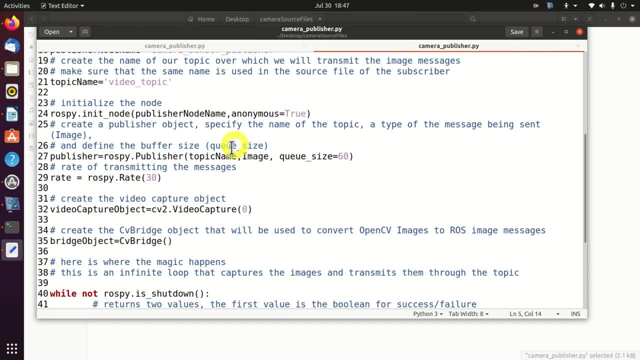 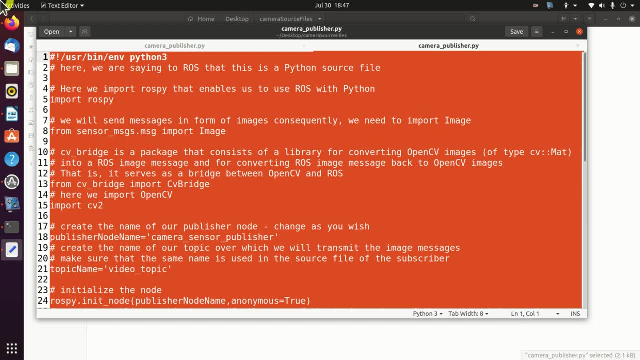 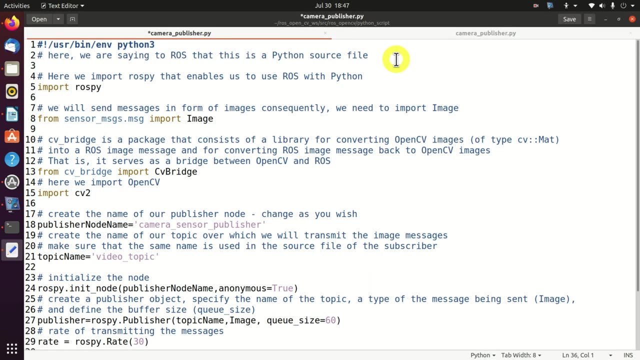 that implements the camera publisher. I will simply copy and paste certain sections of this file. Here is the first part. Let's explain the first part Over here. I'm saying to Ross that this file is a Python source file and every source file that you will write in Python should. 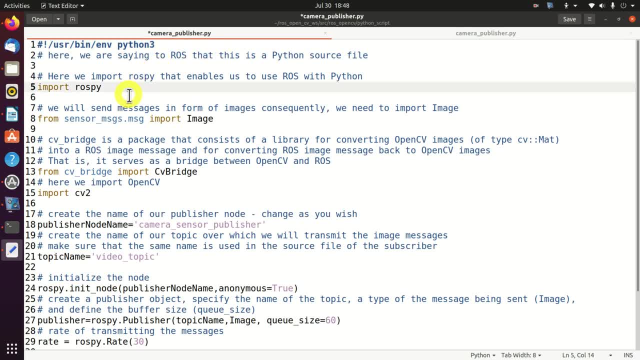 start with this simple line. Next, we need to import Rosspy that enable us to use Ross with Python. Then, since we will send image messages over our topic, we need to import images. Here it is. Next, we need this package and this library. cv-bridge is a package that 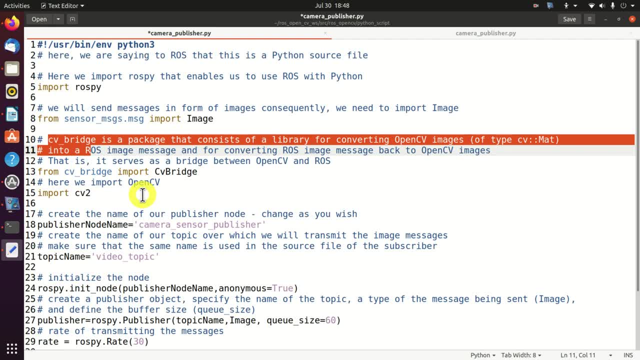 contains a library for converting OpenCV images into Ross image messages and for converting Ross image messages back to the OpenCV images. That is, this package serves as a bridge between OpenCV and Ross. Consequently, we need to import this package and library. And finally, we need 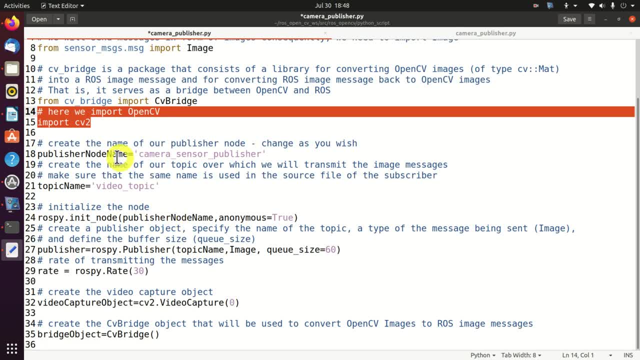 to import OpenCV. Next, we create the name of our publisher node. I call the publisher node camera sensor publisher. However, you can use any other name. Then we need to make the name for our topic. I called the topic video topic, Of course. 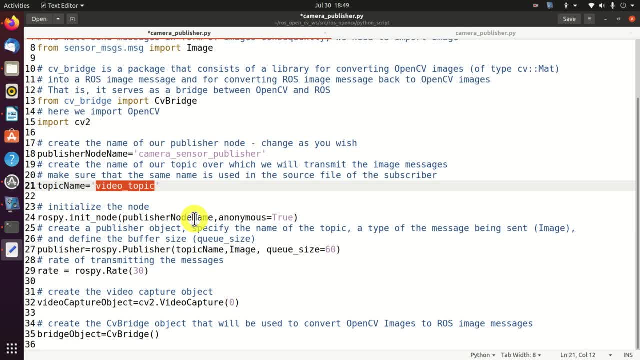 you can change this name as you wish. Next, we need to initialize our publisher node. To do that, we use this function init node and over here we specify the node name that's defined over here, And then we specify this parameter to true. This means that Ross will add a random 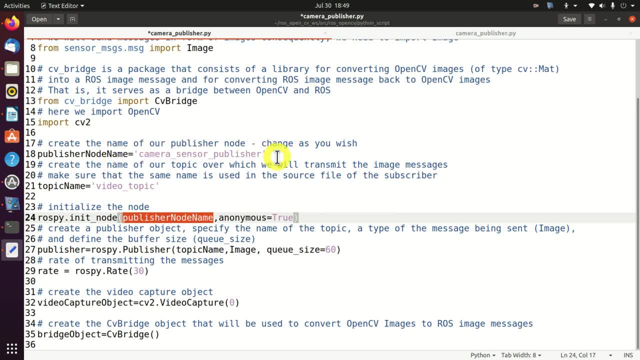 number to this name in order to avoid name conflicts. That is, it will make sure that we always have a unique name for our publisher. Next, we need to create a publisher object, specify the name of the topic and specify the type of the messages that will be sent, and define. 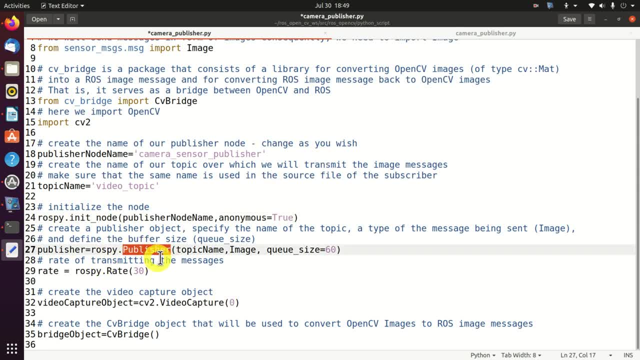 the buffer size. We do that by using this function. We specify the topic name, We specify the data type of the message that we will be using, That is, we will transmit images over our topic, and we define the buffer size, The buffer size. 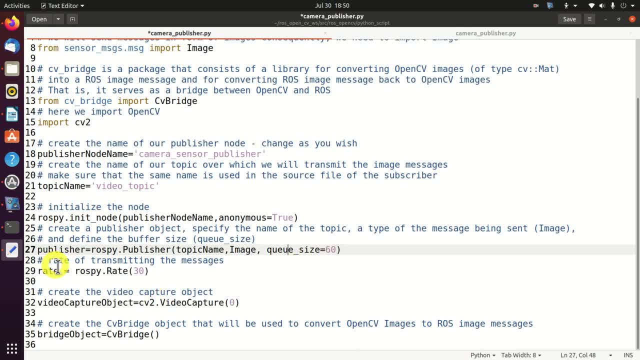 is equal to 60.. Next we define the rate of transmitting the messages. We will transmit the messages or images with 30 Hertz, That is, 30 messages or images per second. Next we call this openCV function, video capture, to create a. 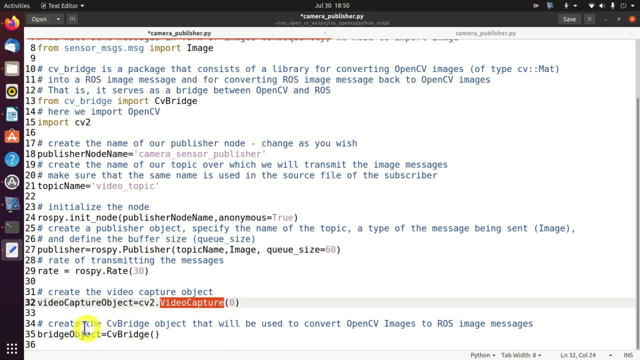 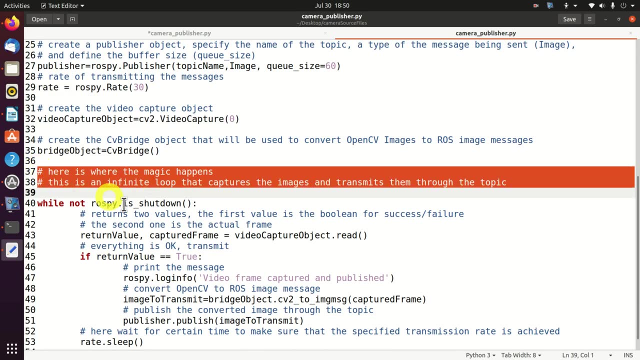 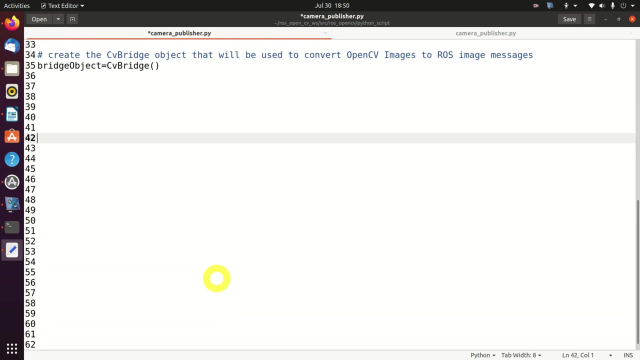 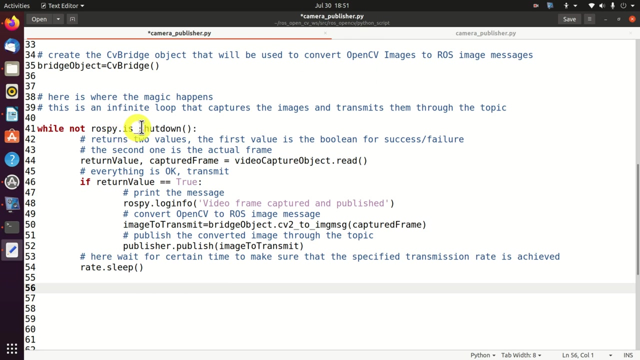 video capture object. Next, we need to create the CVBridge object that will be used to convert openCV images to Ross image messages. And that was the first part of the code. Let's explain the second part of the code. Here is where the magic happens. This is an infinite loop that captures the 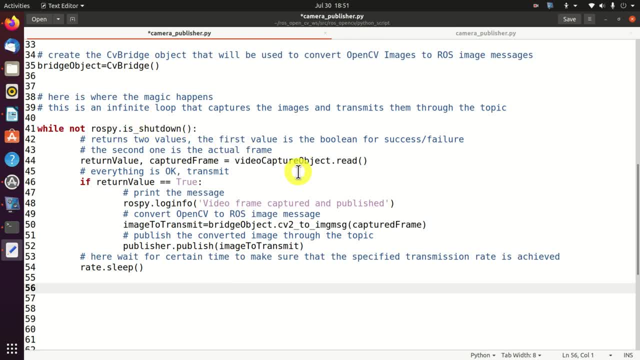 images. converts images from openCV form to the form that Ross can understand and transmit these images in the Ross form to our topic. First we call this function read: This function will actually capture the image and it will also have another value called return value. that will be a. 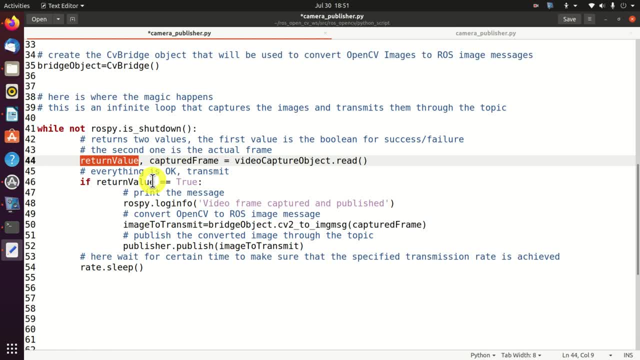 boolean indicating success or failure. If everything is ok, we need to transmit. So if the return value is ok or true, we print the message Video frame captured and published. Ok. next we need to convert OpenCV image, that is, this captured frame from the openCV form to the Ross form. 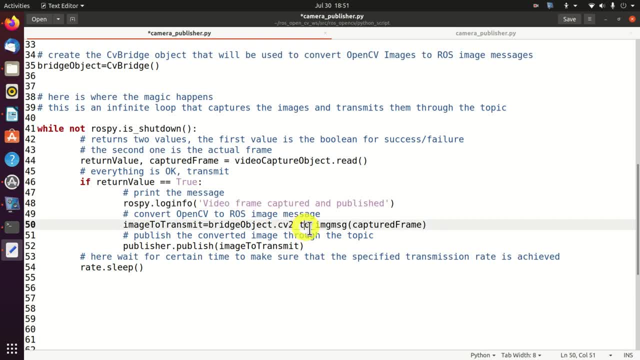 And for that purpose we use CV to image messages function, and this function is basically a method of this object bridge object and bridge object is constructed over here. Ok, we specified the captured frame And this return value will be an image in the Ross image form or Ross image message. 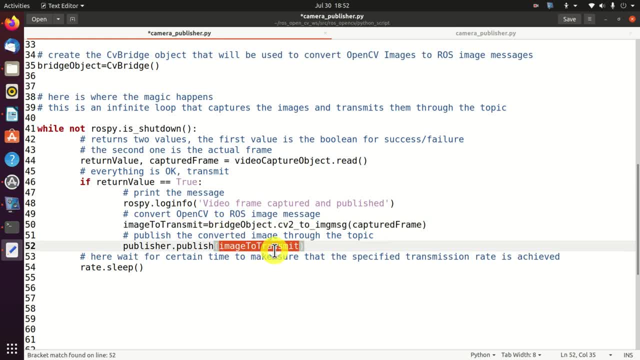 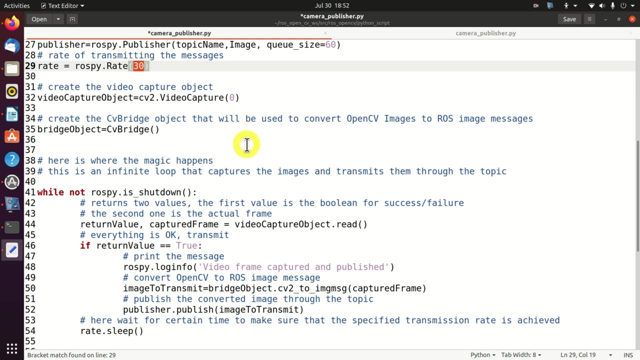 form And finally, once we do that, we transmit that message to our topic And at the end we wait for certain amount of time to make sure that we transfer the image with the specified rate, and the rate is 30 Hz over here. Next, 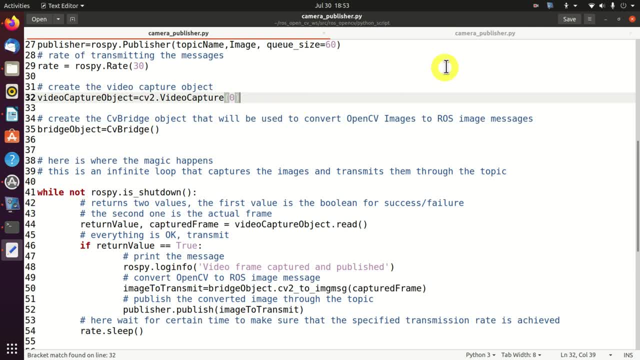 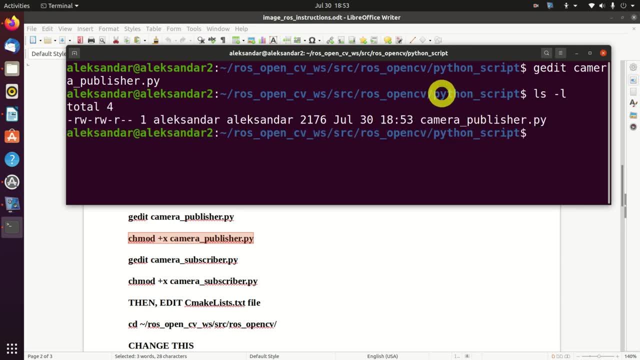 Save this file by pressing control S and let's close this window. Let's go back to our terminal. Let's see the structure of our folder. Aha, we see our camera publisher over here. However, there is one issue: We cannot execute this file since we don't have X over here. 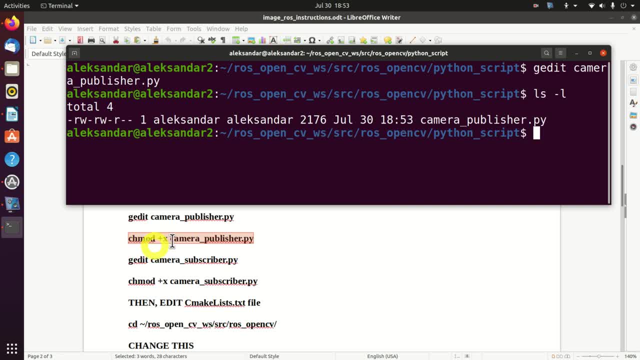 So we need to change a few things. We need to specify that this file is the executable file, And we need to add this parameter. So let's do that by using the command chmod and let's see the result. Here it is: We have now the file that can be executed. 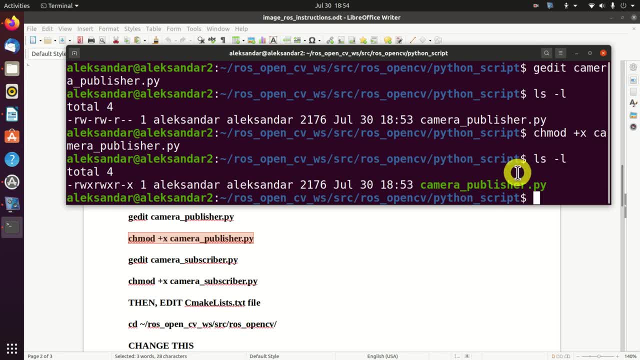 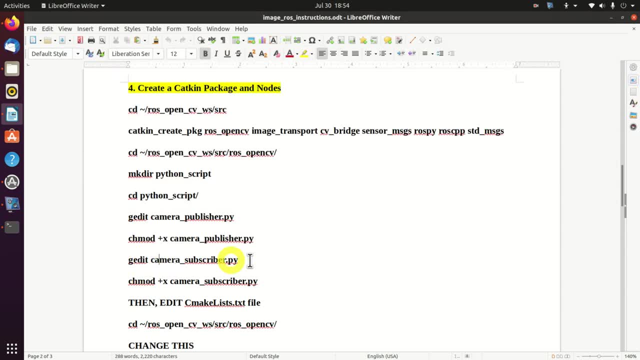 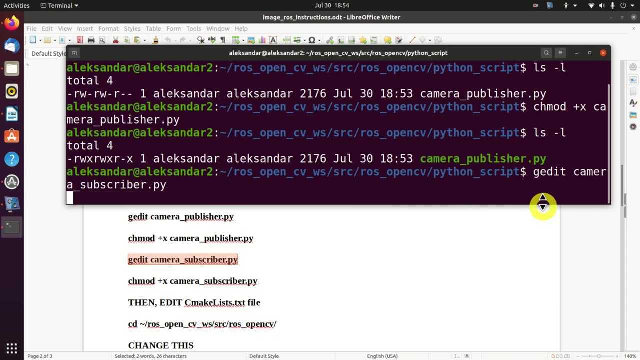 Next, let's create the subscriber node, That is, let's create its source file. Again, I will be using geditor and I need to specify the name of the file, So let's do that. Ok, Here we need to type the Python code. 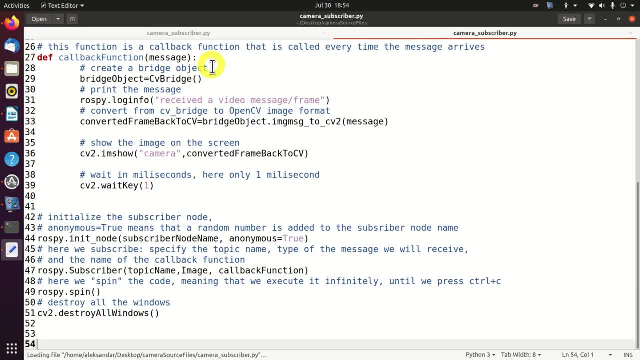 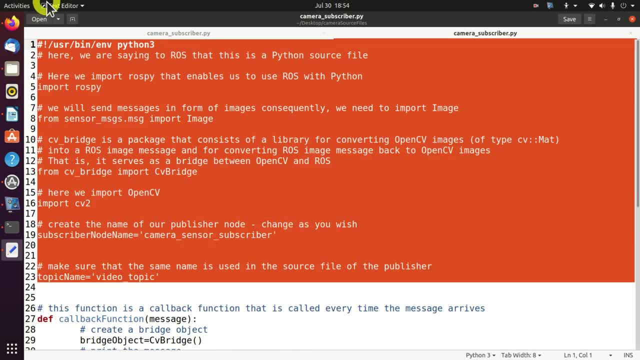 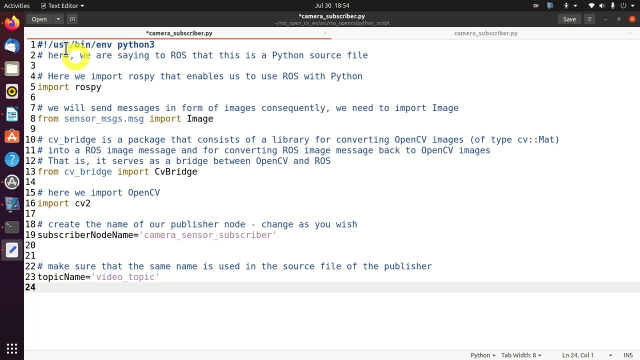 However, to make this video as short as possible, I will simply copy and paste the file that I previously wrote. Let's first copy and paste the first part of the file. Let's see what happens over here. Here again, we are saying to ROS that this is a Python source file. 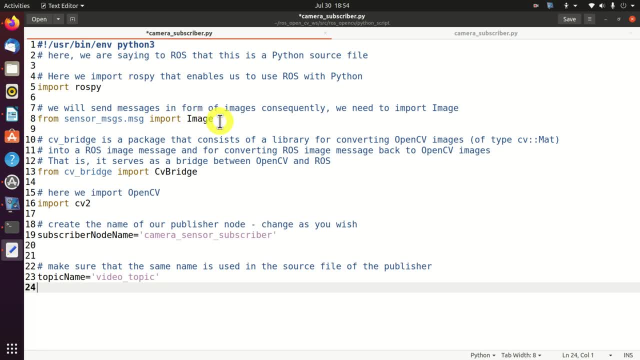 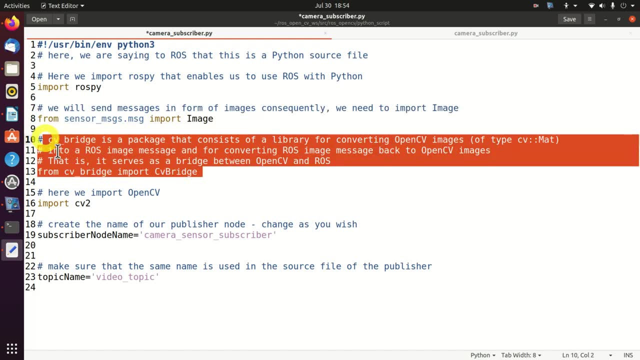 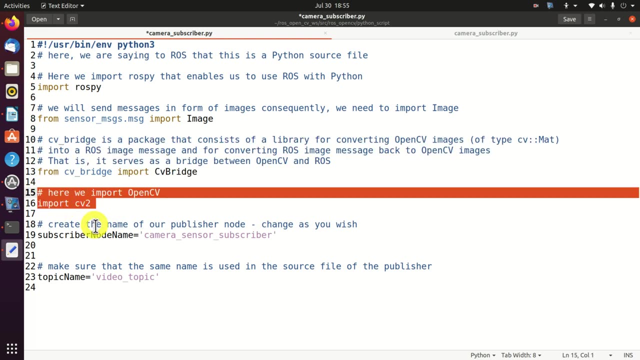 Then we need to import ROS And, of course, since we will be receiving images, we need to import image. Then we will be using cvbridge to convert from OpenCV to ROS formats And we import OpenCV. Next we create the name. We give the name to our subscriber node. 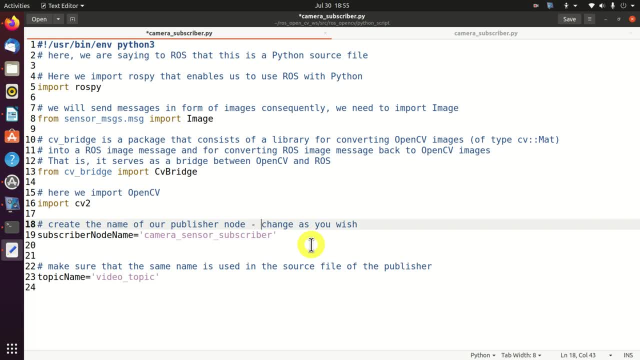 I call it camera sensor subscriber. However, you can change this name if you wish. And over here we need to give the name to our subscriber node. And over here we need to give the name to our subscriber node. And over here we need to give the name to our subscriber node. 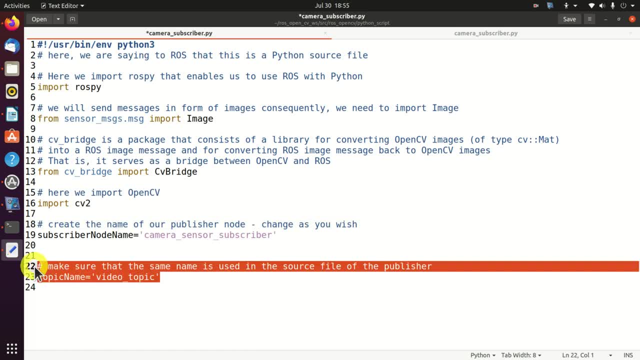 I call the topic as video topic Here. you should stop for a second and make sure that this name completely matches the name of the topic name in our publisher node. If that is not the case, this code will not work. Ok, Let's continue. 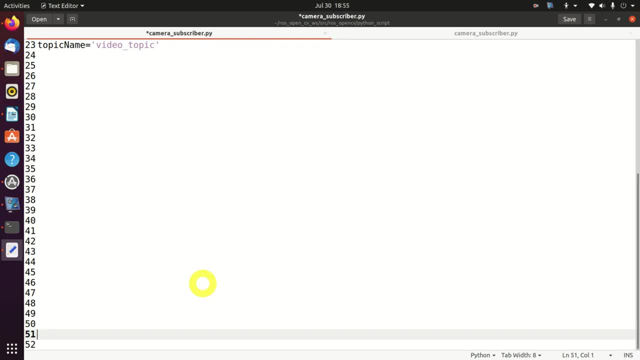 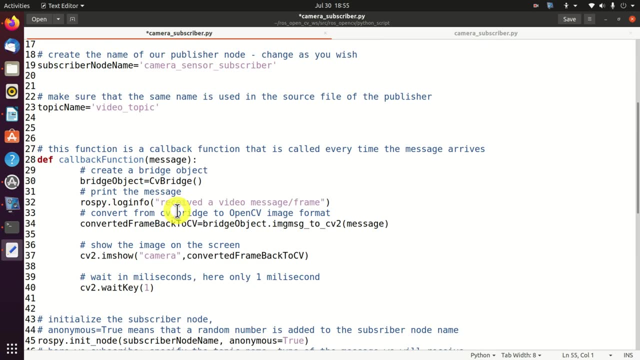 Next I will paste the second part of the code here it is. first we need to define a callback function. this callback function is called every time the message arrives to our topic. the callback function accepts our message. that is the image. then we need to create a bridge object. 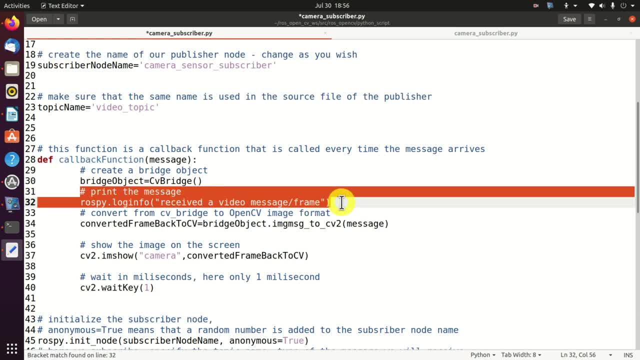 then we need to print the message saying that we receive the video message and frame and over here we need to convert from CVBridge form to OpenCV image format. consequently, we will take the message and the message is in the ROS image format and we convert this image by using this function, to the image that. 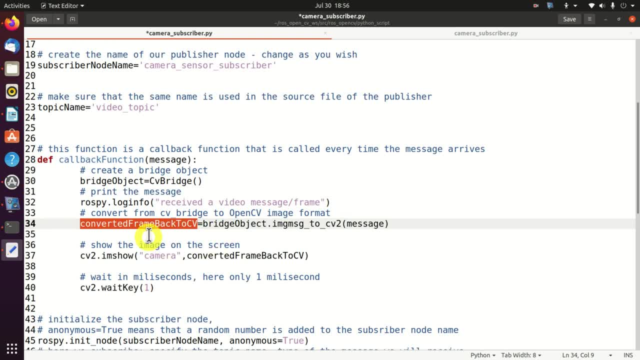 is in OpenCV form. after we do that, we simply show our image on our screen. okay, so now we have our image on our screen. so now we have our image on our screen. so now we have our image on our screen. then we wait in milliseconds, for example, only one millisecond over here. 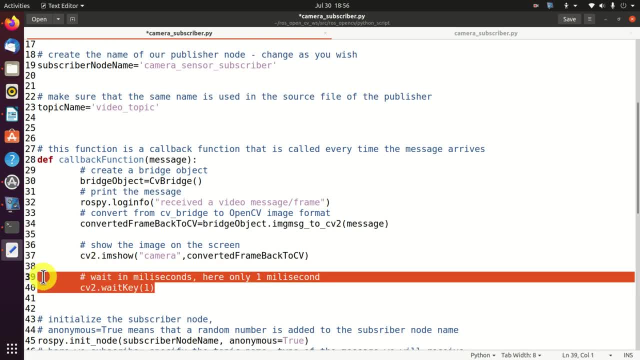 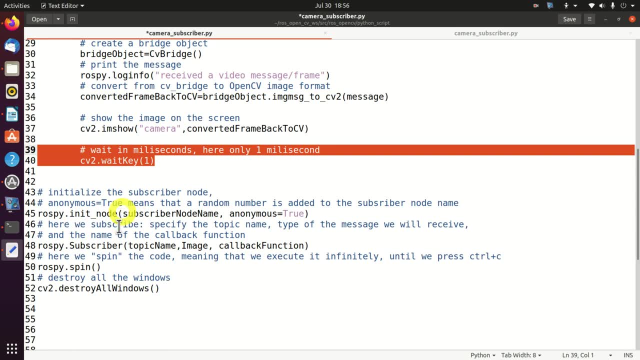 for the frame and an image to refresh on our screen. okay, that was our callback function. next, we need to initialize our subscriber node. we use this function, we specify the node name that's previously defined and the next thing is to tell to ROS that we want to subscribe to our subscriber node and we want to subscribe. 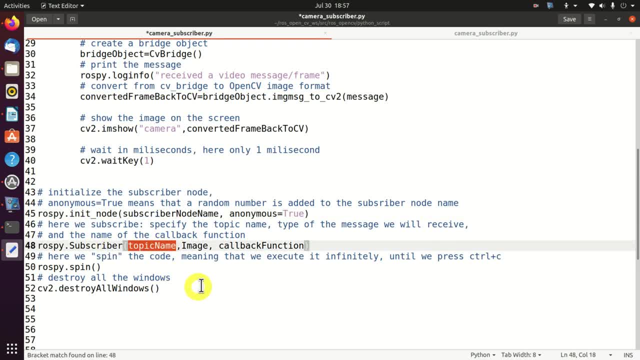 to our subscriber node and we want to subscribe to topic. here is the topic name. this is the first to topic. here is the topic name. this is the first argument. the second argument is the data type we argument. the second argument is the data type. we expect to receive images and consequently over. 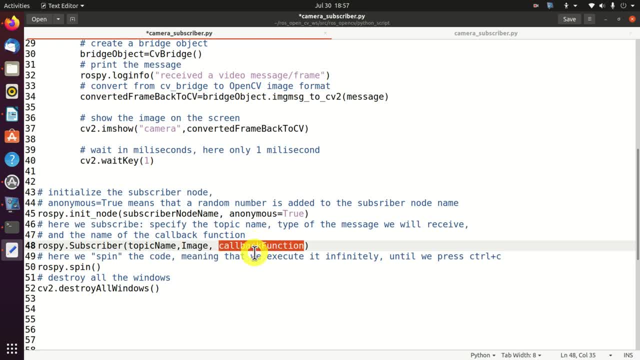 expect to receive images and, consequently, over here we have image and we specify the callback. here we have image and we specify the callback function. so what's happening over here, once the function, so what's happening over here, once the image is being transmitted to our topic, we call. 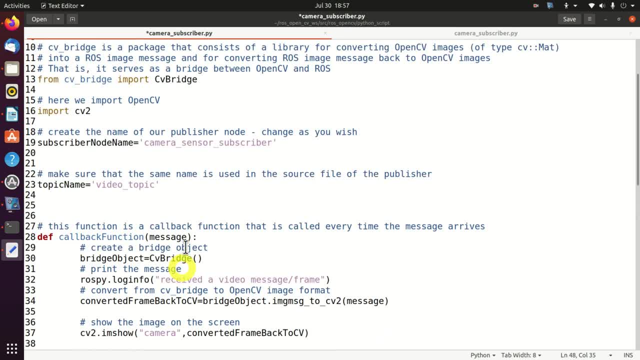 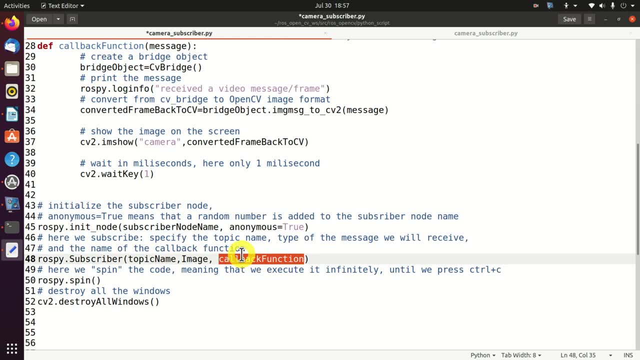 image is being transmitted to our topic. we call the callback function. the callback function will. the callback function will take that image, convert image from the ROS form to the OpenCV form and show the image on our screen. okay, finally, we need to spin the code. this function basically serves as the while loop. it will simply run this code and 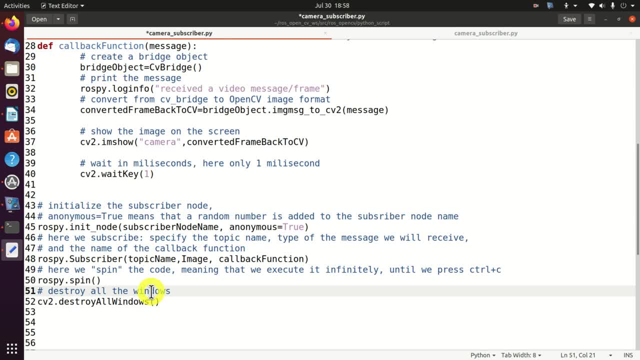 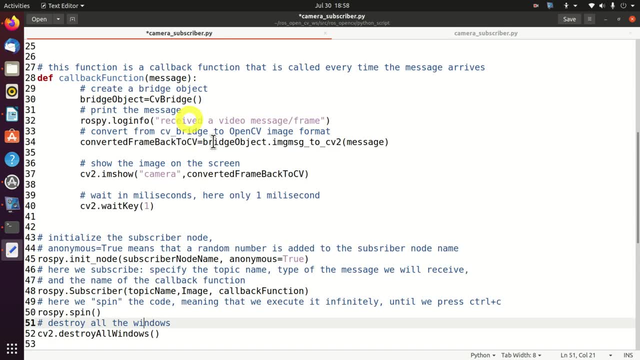 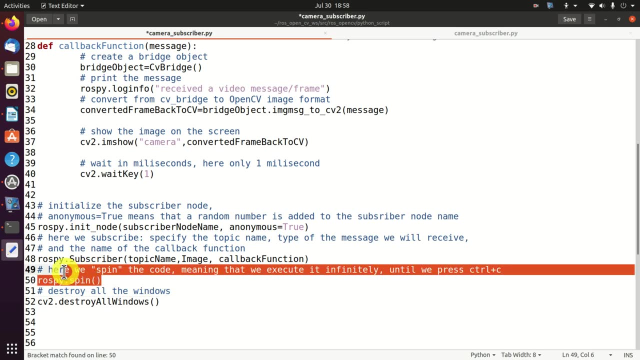 run it and run into run it. basically what will happen? this code will wait until the image shows. once the image shows, this callback function will be called, this piece of code will be executed and again, we will wait until the next image arrives. if you press ctrl C during the execution of this code, 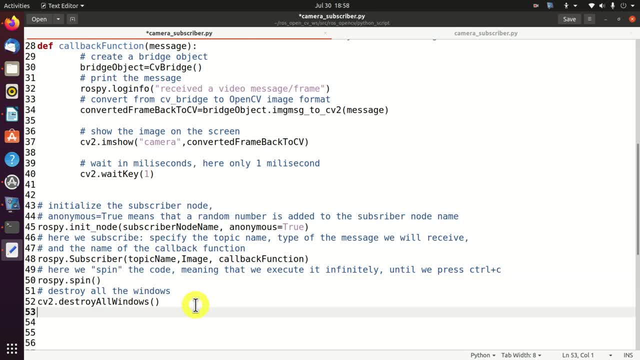 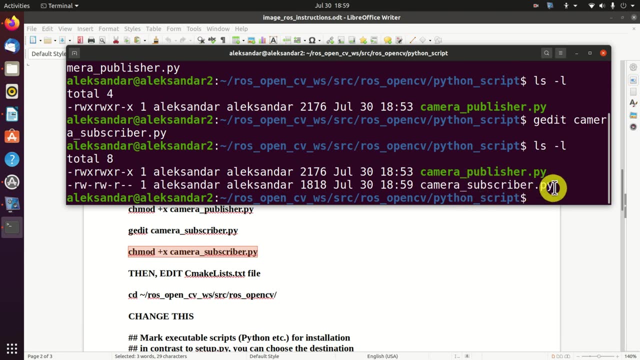 this function will return. and finally, we need to close all the windows. so that was our subscriber note. next, we need to save this file, close this window. let's go back to our terminal. let's see our file. here is the note that we created. however, again there is an issue with an X is over here. that is. 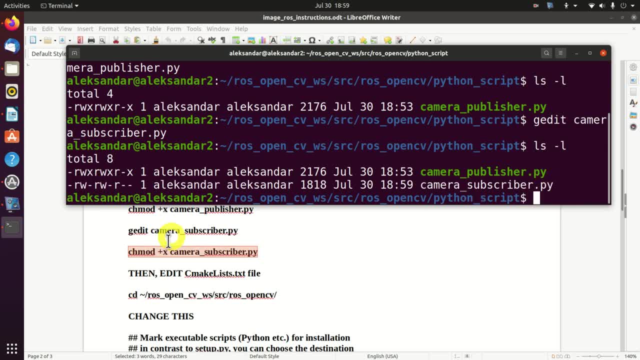 you can see that we have created an error here, so we need to go back to our terminal. let's see our file. here is the note that we created. however, again, there is an issue with an X is over here, that is, we cannot execute this file. consequently, we need to type CH mode plus X. 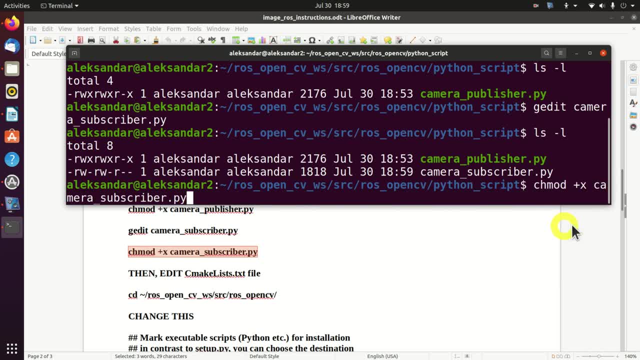 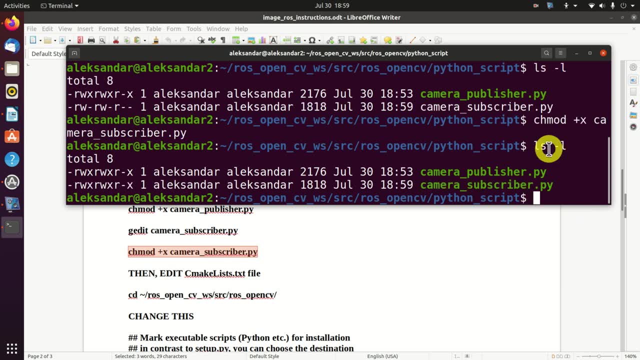 and camera. subscriber: dot PI. let's do that. here it is. let's verify that everything is correct. aha, perfect, we can execute both of our nodes. however, we still need to perform one important step. currently, our Ross and our CMake environment cannot recognize where the source files. 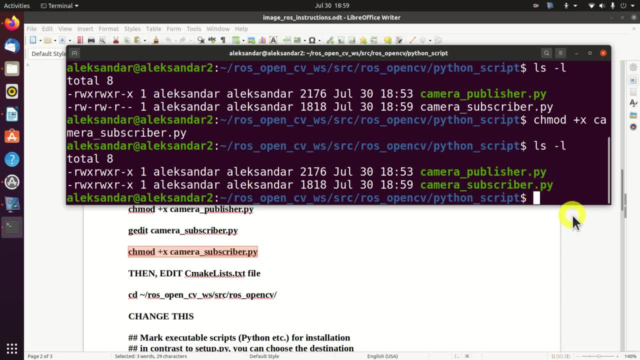 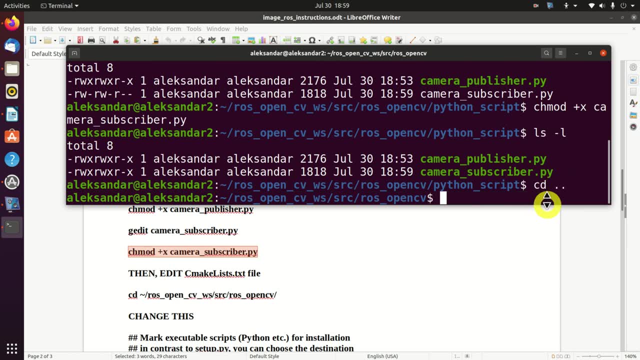 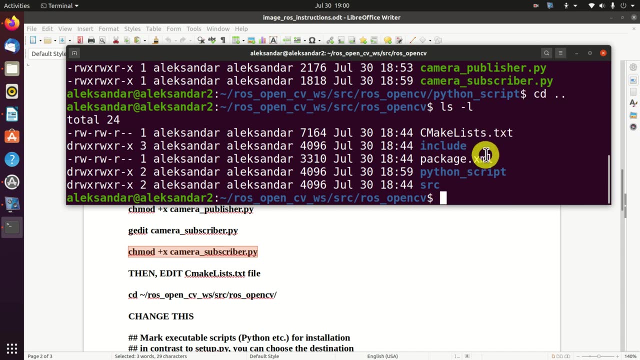 although they are here. we need to somehow tell to our CMake and Ross that the source files at are at this folder. to do that, we need to go one folder back and we need to edit this file: CMake lists. let's do that to edit this file. we. 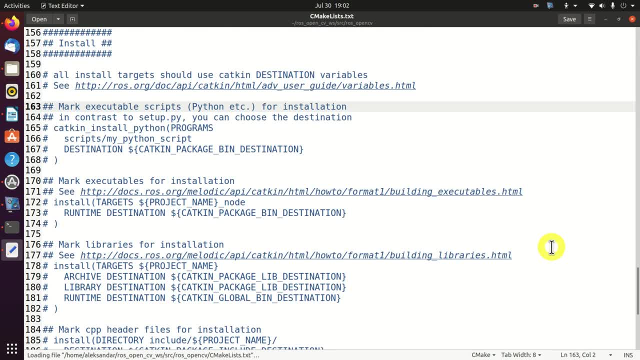 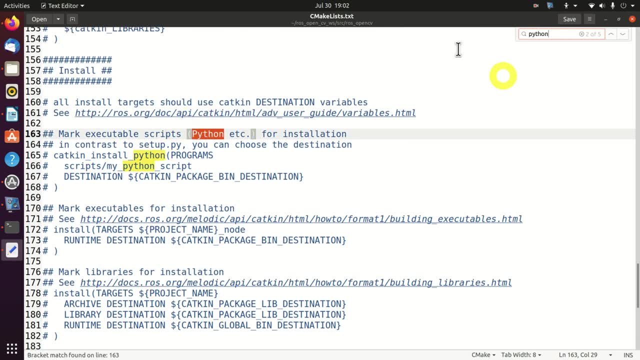 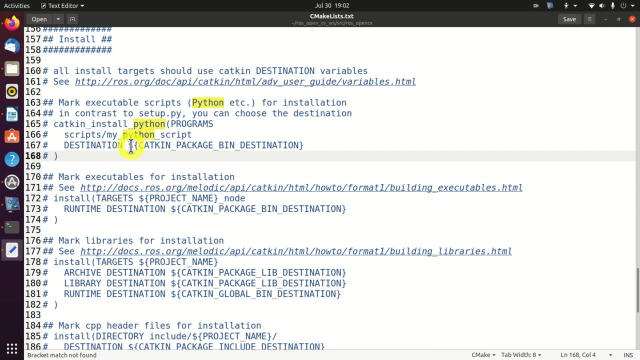 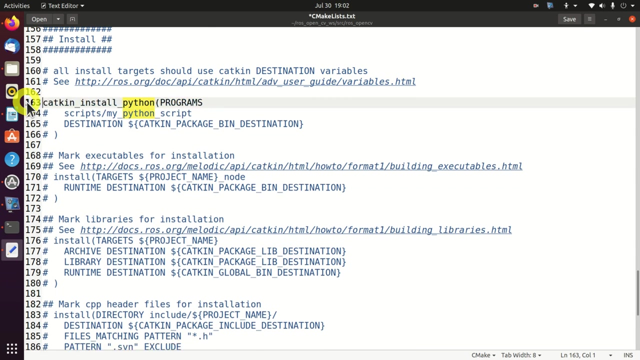 will type this command, then search for Python. if you start searching from Python, you will start from here. then here's the piece of code that we need to change. first of all, I will erase these comments, then I will uncomment these four lines. the most important modification is given. 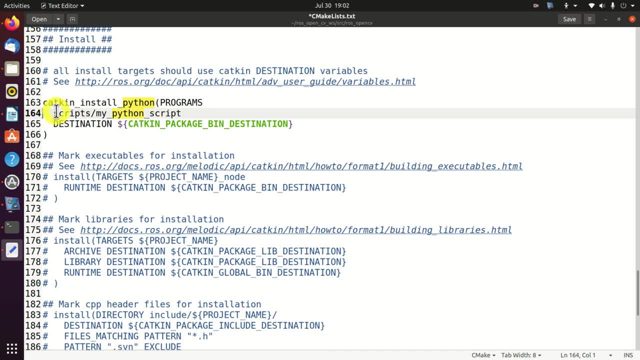 over here. here we need to specify the path to our source files. in our case the path is different than the path given over here, so let's correct that the name of the folder is Python script. consequently, over here I will modify this part: Python script. and over here we need to specify the file names, the name. 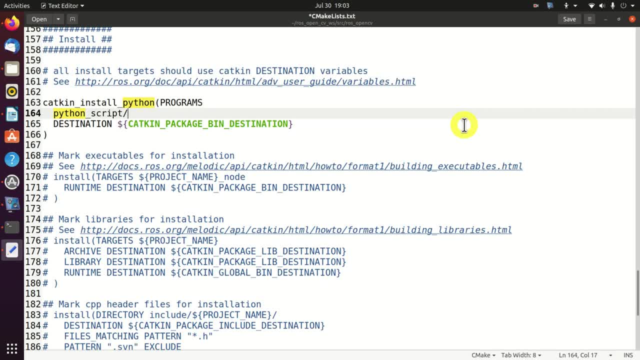 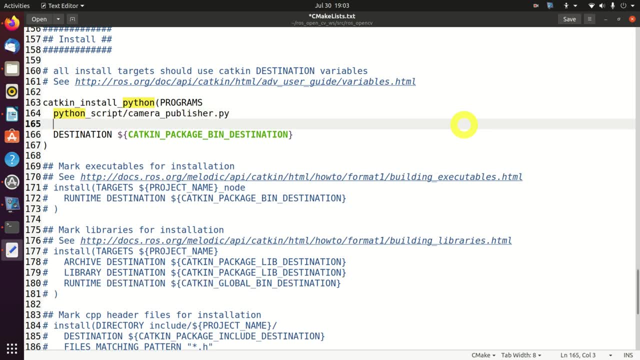 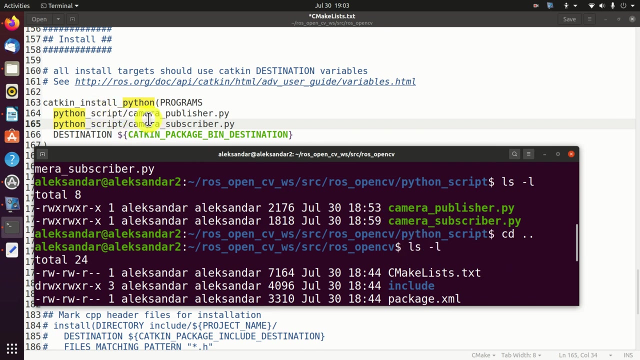 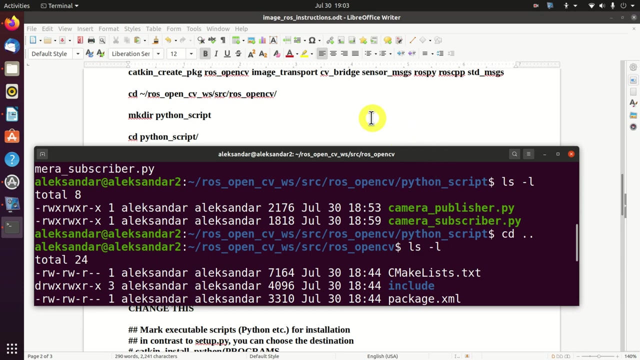 of the first file is camera publisher, dot PI. camera publisher. the name of the second file is camera subscribed or PI, and over here we need to verify that the names are correct. Python script- Python script- camera publisher, dot PI. camera subscriberpy. so far, so good. save this file, exit and let's perform the next step. 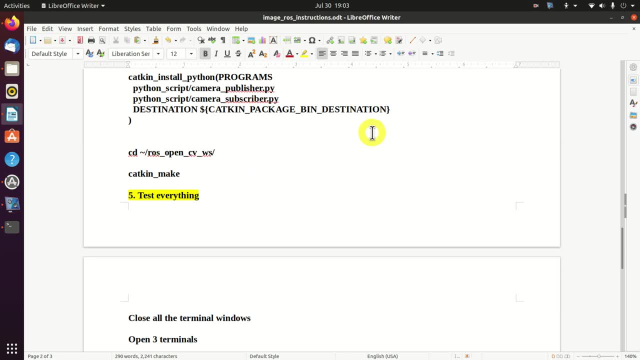 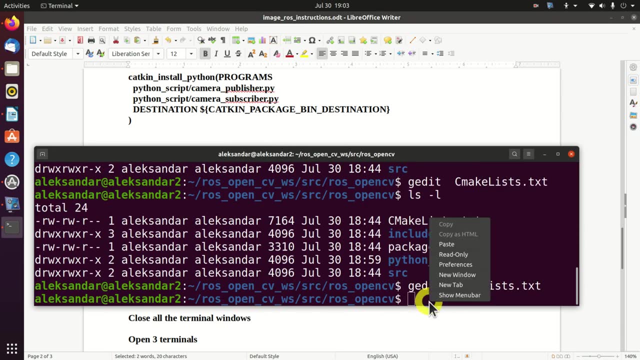 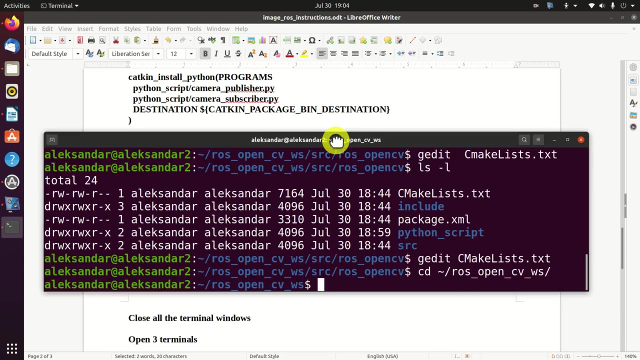 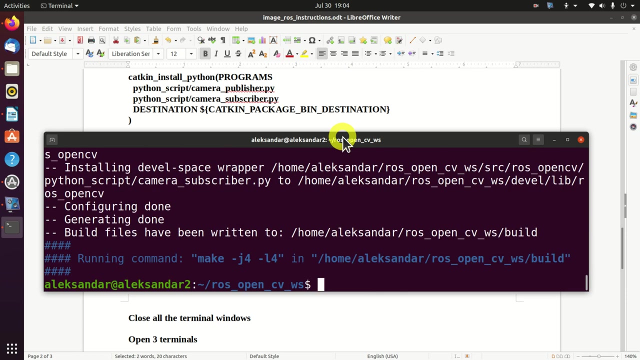 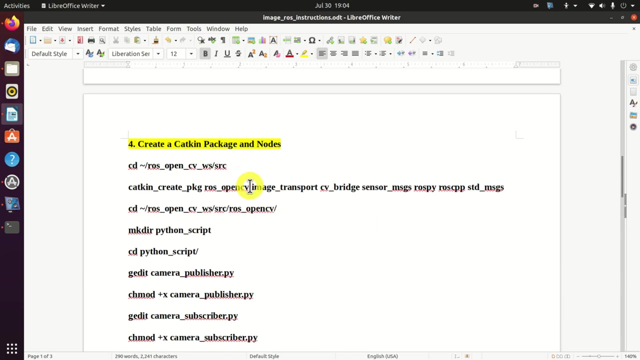 in the next step, we need to run catkin make. however, before we do that, we need to go to the appropriate folder and inside of this folder, we need to type catkin make. okay, so far, so good. now we have completely created our package, and the next step is to test this package. 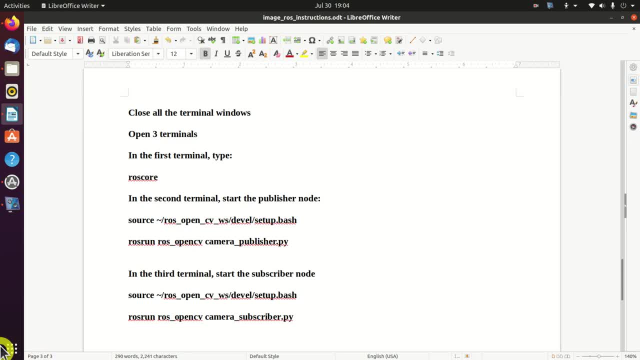 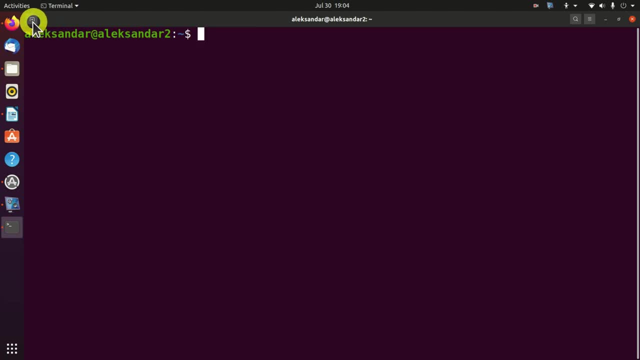 let's close everything and let's start from scratch. open a new terminal and, in addition to that terminal, open two new terminals. by clicking over here, in the first terminal, we will run our ross core, that is, we will run the ross master that governs.